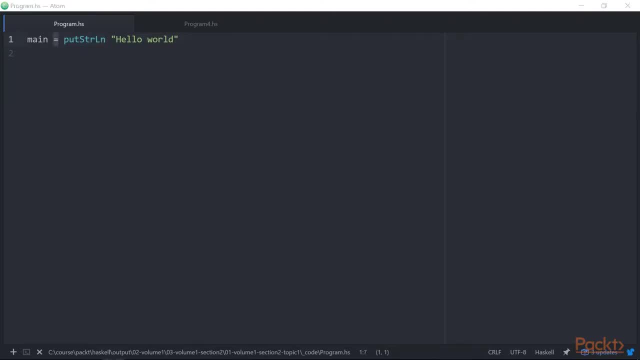 within an expression on the right hand side of the equals sign. The equals sign is the operator and this is the type or value naming operator and is either pronounced equals or is. And thirdly, we see the string literal delimited with double quote characters. Thus: 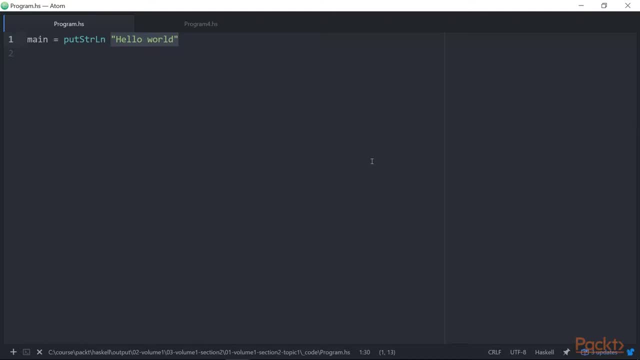 this declaration can be pronounced as: main is put: strln. hello world. Semantically speaking, this program binds or assigns the name of the string literal to the string literal. The string literal is the name of the variable main before the equals sign to the expression. 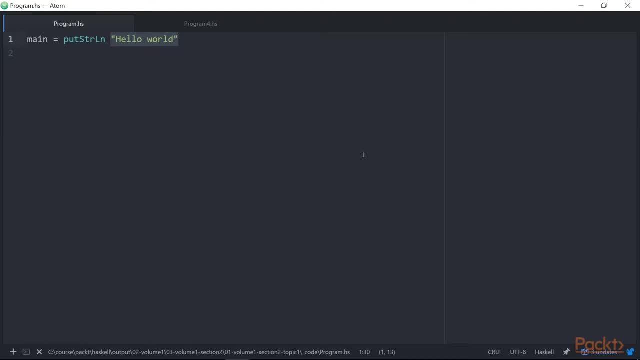 put strln- hello world. on the right hand side of the equals sign. This right hand side applies the function put strln to the argument hello world. Put strln is a function that takes a single argument of type string and evaluates to an action that, when executed, will print the string to the terminal and produce no result. Haskell's. 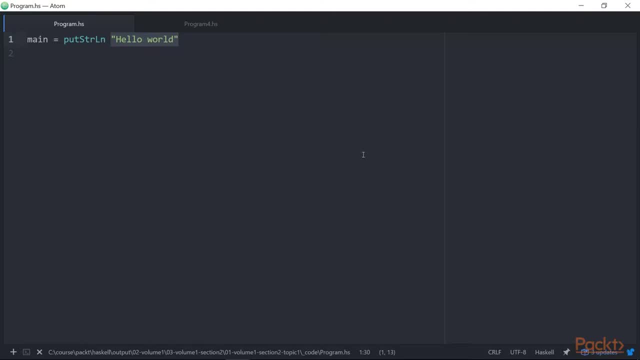 standard string type is a list of unicode characters. Thus main itself evaluates to an i-o action that produces no result, And when this action is later invoked or executed, it will print the unicode characters hello world. to the terminal. Let's figure out how to run this program. We'll be using stack, so I've created a stackyaml. 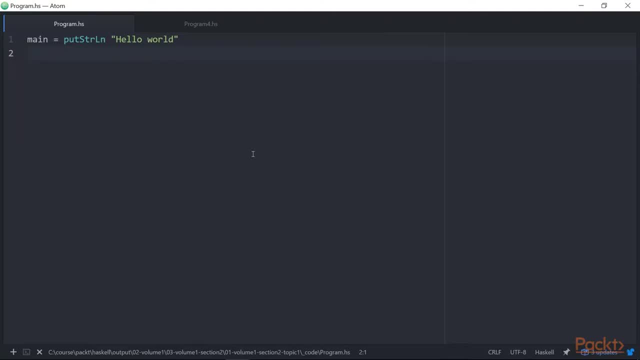 configuration file in the same directory as the source file to tell the stack command which resolver to use. As specified in the installation and setup guide for this course, we'll be using the LTS 7.8 resolver. I'll talk more about that later And furthermore, 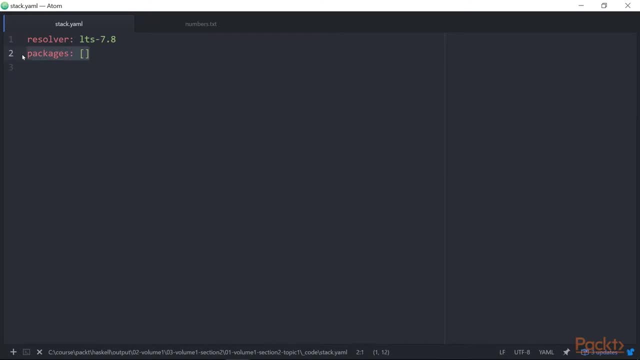 we're not going to reference any packages other than the standard base package. So there's an empty list of packages, And base is Haskell's standard library that is, by default at least, available to all programs. So we'll open a terminal and we're going to use stack's runghc command to quickly. 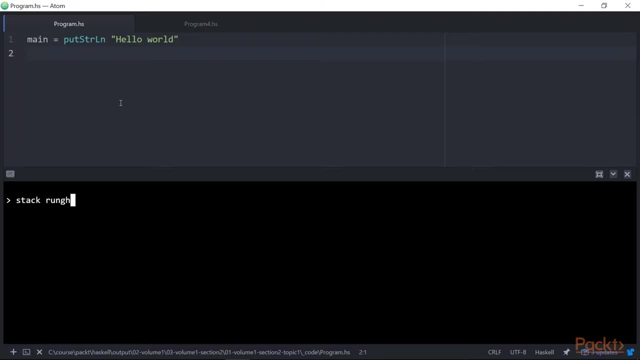 run the program stack runghc programhs, And there you go. it does exactly what you'd think. This program will be fully type checked and have unambiguous types assigned to each element before the program is run. Furthermore, the language specification is such that it doesn't matter whether this is 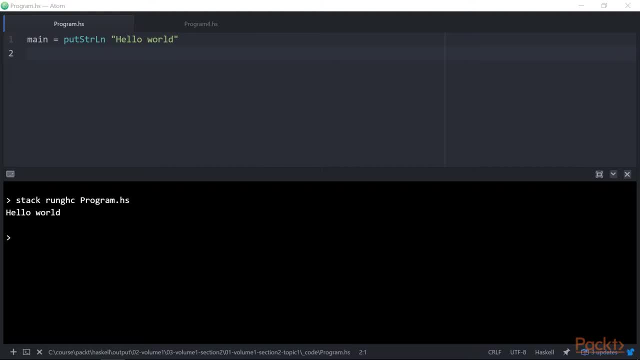 done by a compiler or an interpreter, The program will still be statically typed and in fact, runghc is an interpreter and runghc is used to quickly and iteratively run programs. So while runghc is an interpreter, the semantics of the program will be identical to those 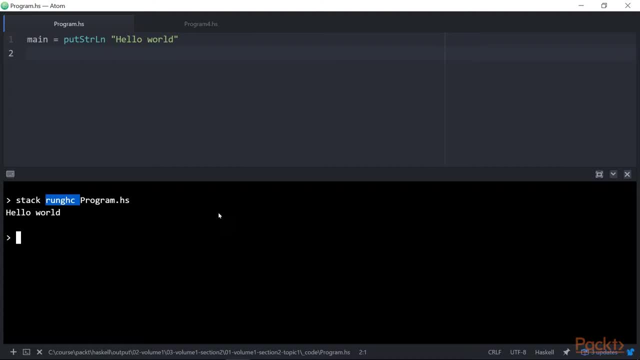 produced using the ghc compiler, using the stackghc command. You can also run here stackghcprogramhs and it takes a little while longer. Haskell does support type signatures and these are optional in most cases and only required in others and typically only required to eliminate type ambiguities. 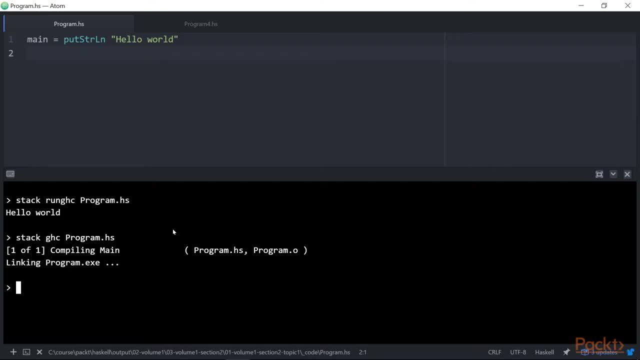 This program does not currently use type signatures, but we can add some in and run the program again. We'll go to the top here, we'll add a new line and we're going to type main Double colon io: open parens, close parens. 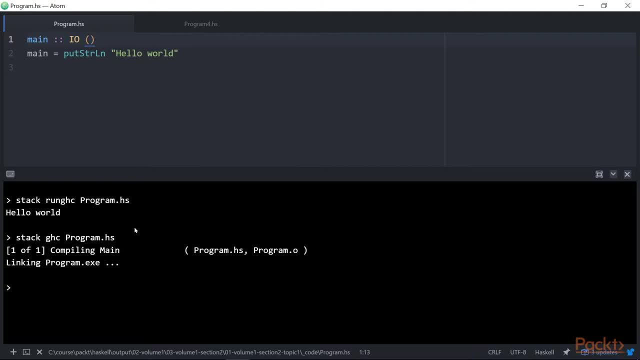 We save the file and we will run it again. It yields exactly the same result. And just to convince you that it really is compiling that program, I can put some garbage into it, save the file and attempt to run it again. 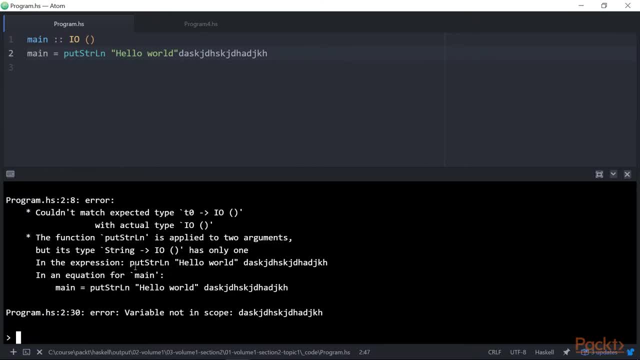 There we go. we get an error message. An expression put strlen: hello world with my garbage. So we'll take the garbage out And we'll look at the type signature again. This uses the double colon operator to specify the type of the name main on its left hand. 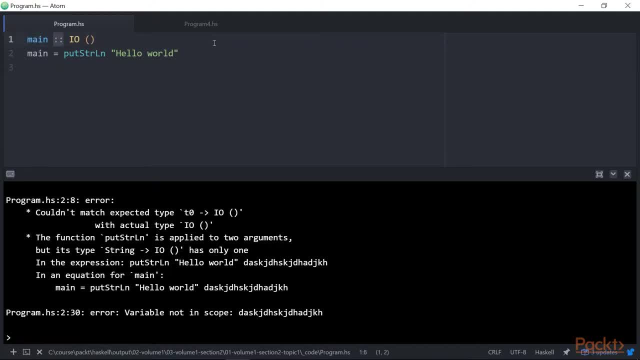 side. This operator is typically pronounced has type. Next in the signature, after the double colon, is io. Io is a type class and is a family of abstract data types representing actions that can be invoked to perform input and output, and we'll talk much more about this later. 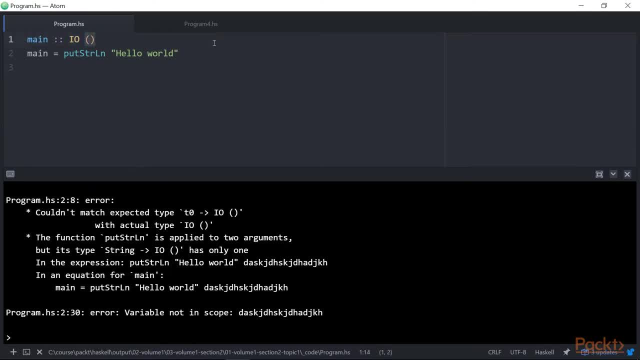 Then we see open and closed parentheses. This is pronounced unit And it is a type containing a single variable, A single value, also named unit and also represented by open and closed parentheses. This unit value is conceptually equivalent to a tuple with zero elements. 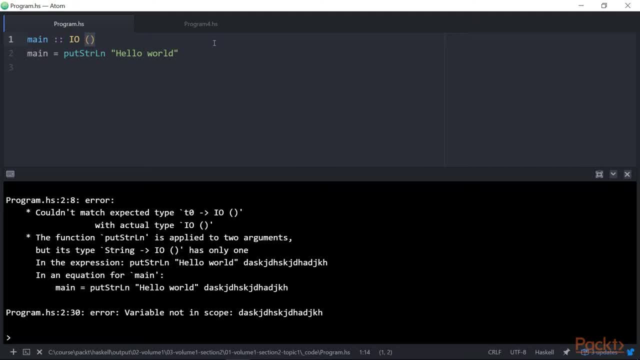 Since the type unit has exactly this single value, it effectively conveys no information Unit is often, though not exclusively, used by io actions when all we really care about are the side effects of the action. And the side effect, in this case, of the particular main function we're looking at here is the 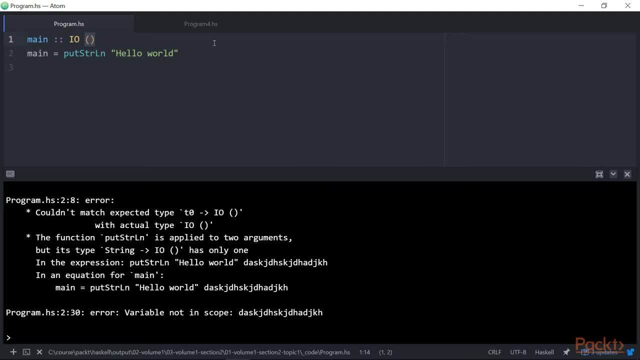 writing of characters to the terminal. It should be noted that there is nothing magic about unit. It should be stored in collections and operated upon much like any other value. Overall, therefore, the type signature is pronounced main- has type io, unit And in English this means that main is a function that evaluates to an io action, which 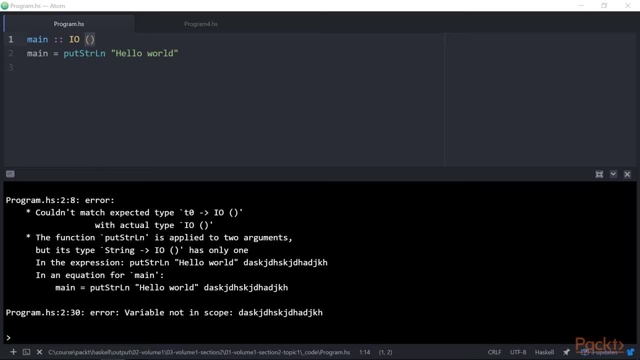 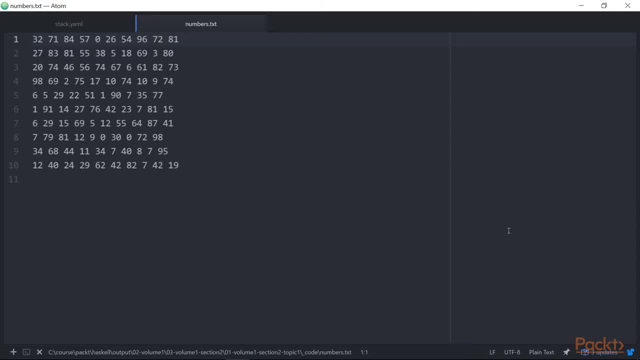 produces no value. Now let's do something a little more interesting. Here I have a text file- numberstxt- and it consists of 100 random integers. So let's go back to our program and we're going to add a do block. 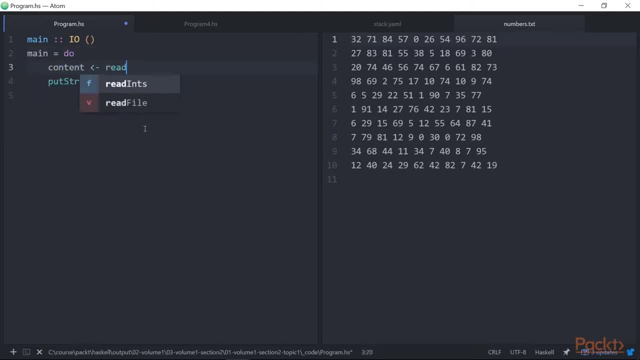 And add another line content from readfile numberstxt, And then we'll modify the last line. to do put strlen on content. This evolution of our little program introduces some additional syntax and references a new function from the Prelude, namely readfile. The Prelude is a standard module that exports a large subset of the functions defined in 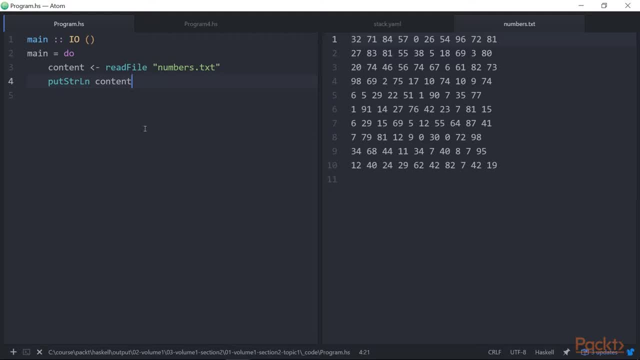 Haskell's base package, The Prelude, typically exports very commonly used functions. The new syntax is a very interesting one. It's a simple one. Syntax is the do here and the left pointing arrow here. The left pointing arrow is pronounced from or drawn from. 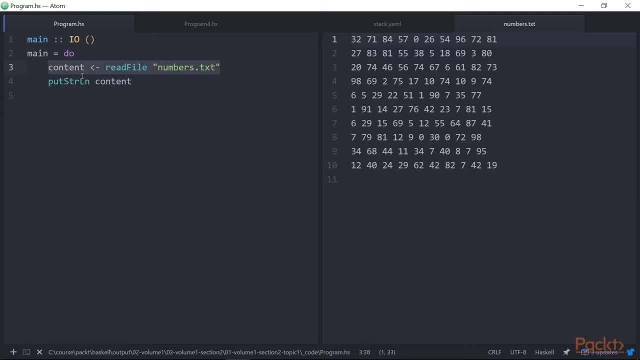 The code is thus pronounced: content is drawn from read file applied to numberstxt. This is do notation and is a syntactic convenience introduced to make working with type classes like IO easier. It is much more general than IO, though this will be its primary usage throughout this. 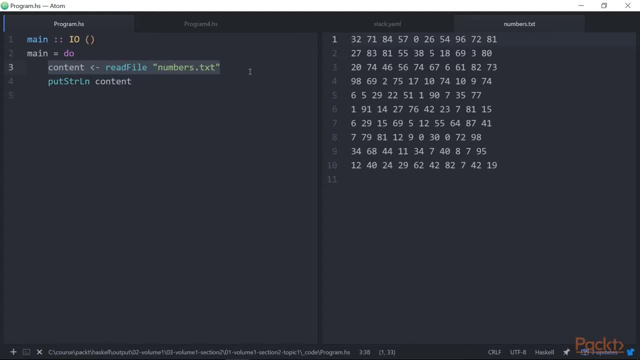 course, Suffice it to say for now that main evaluates to an action of type IO unit. It is the sequential combination of two other IO actions, The first, using read file, applied to numberstxt, highlighted here. This is the IO action that returns the contents of this file as a string extracted using the. 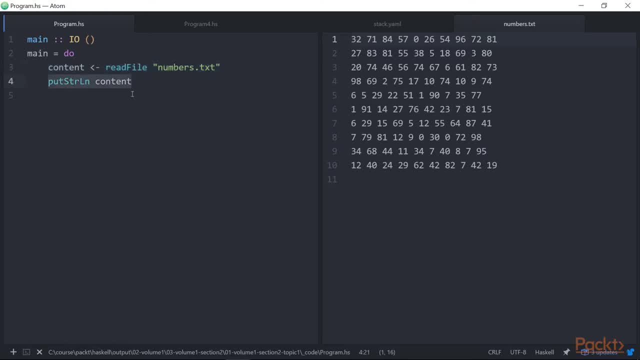 drawn from operator. The second action is the action resulting from applying put strlearn to content, where content is the value yielded by the previous read file. The type of read file is file path maps to IO string, Ie when applied to a file path, it evaluates to an action that produces a string. 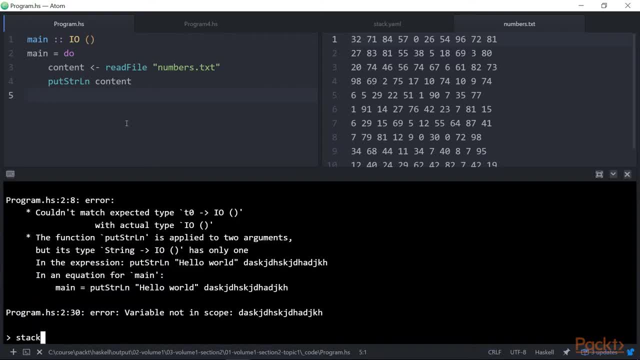 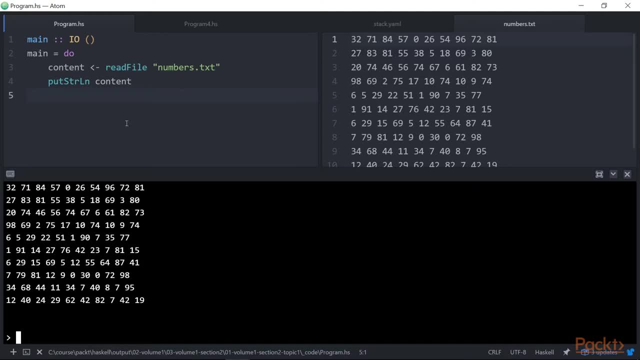 Let's run this program: dac run ghc programhs. There we go. It simply dumps out the contents of numberstxt. Let's also take a look at the print function. Here we are using put strlearn. We can use print instead. 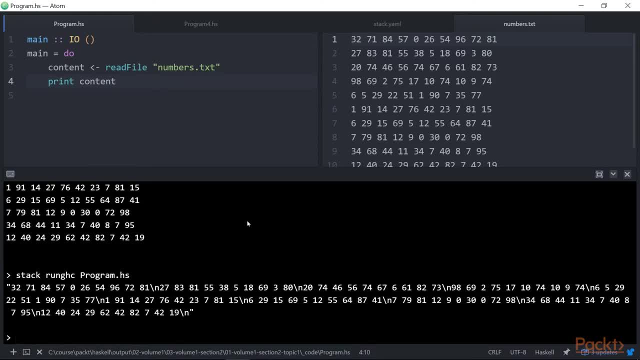 Let's run the program again. Let's observe how the output is slightly different. Put strlearn is used to output a string followed by a newline character. Print instead can be applied to any value that implements the show type class and is typically used to display a representation of a value for diagnostic purposes. 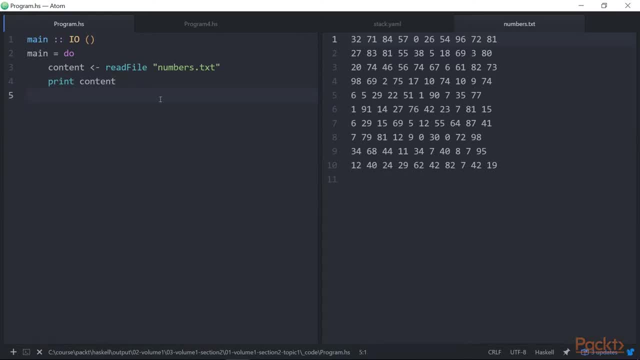 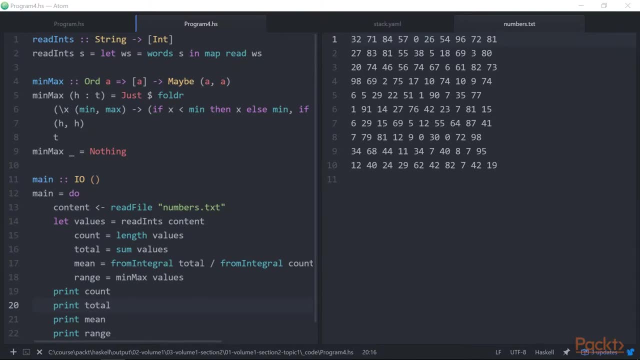 At this point we are ready to really go for it. Close the terminal. I'm going to open up program4.hs. Here is a development of our single program, extended to report various statistics about the values contained in the file numberstxt, As well as introducing two new top level functions, readInts and minMax. this program demonstrates: 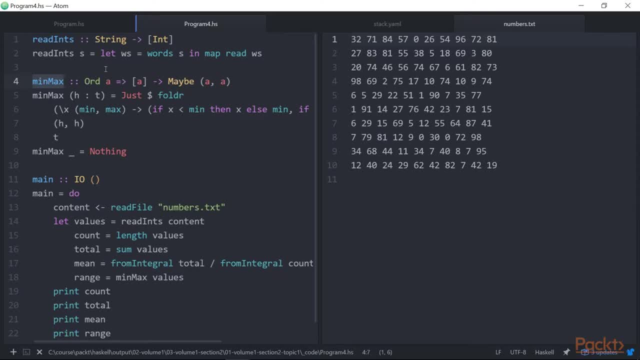 a number of other new things. We see a few new functions from Haskell's standard prelude and in particular in this program we see mat, which we've seen before, a higher order function that applies a function element-wise to a list and yields another list. read: this is a polymorphic function. 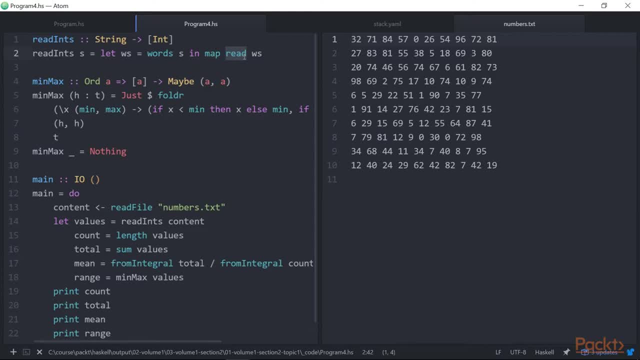 which reads values of any type. that implements the read type class function. For example, it's a list. This is a function that takes a string and splits it on white space, word boundaries, Folder: this is a higher order function for a reduction that we've seen before. 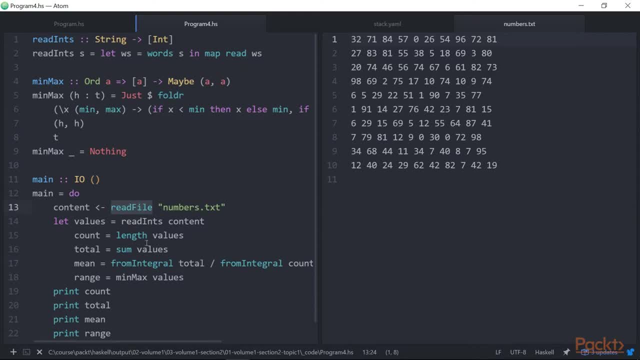 It's a function that reads file Length. this is a function which evaluates to the number of elements in a list Sum. this is a function which evaluates to the sum of the elements of a list of numerical values And from Indiana integral, which converts an integral number to another number. With the same function. we see a low order function which reads values of any type. We also see some functions where the same number of elements in a list is 있고. This is a function which evaluates to the sum of the elements of a list of numerical values. 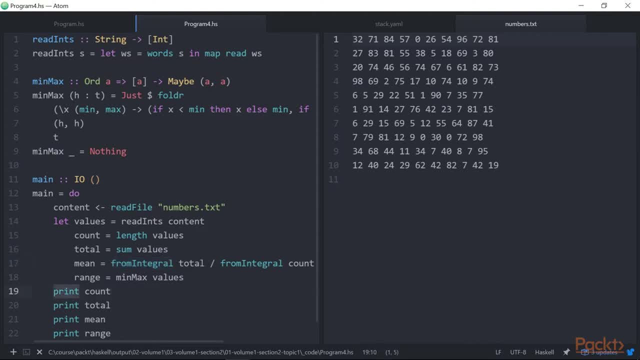 numeric type. Of course we've seen print before. We also see some new operators, most of which are just functions exported by the prelude. Double right arrow, pronounced, implies: introduces a type constraint into a type signature. Right arrow here here is pronounced maps to and is using type signatures. and. 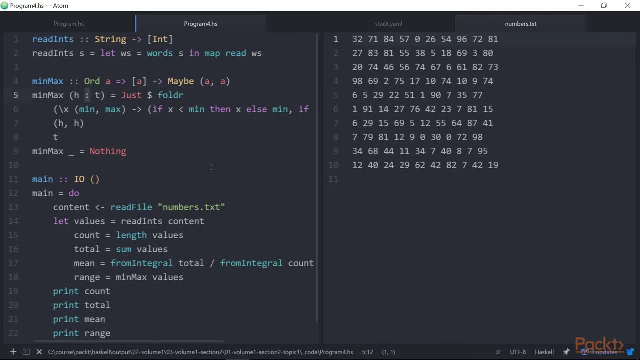 anonymous functions. Colon here is pronounced cons, and this is used to construct a list from a new head element and an existing tail, or, in this case, to pattern match against such a list, to deconstruct it to its head and its tail. We also see less than and greater than, which have their usual. 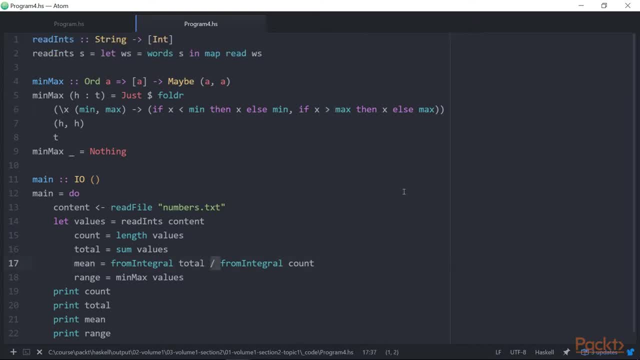 meaning Down here we have divide. Let's look at readints. Readints has a let binding. This introduces the new variable W's- Ws, pronounced W's, It's more than one W and this is words applied to the function argument S and. 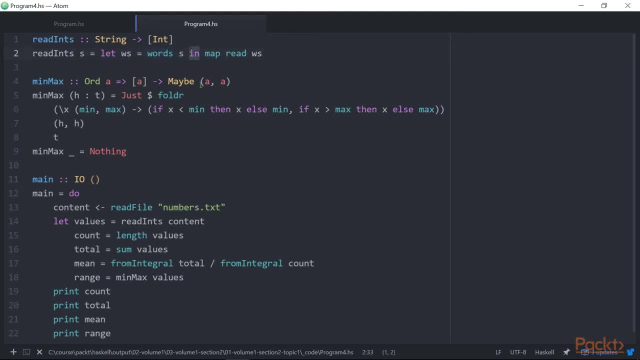 this introduces the name Ws into the expression map. read Ws: Ws to the right hand side of the in keyword. Together these produce a function which splits a string on word boundaries and then applies the read function to each substring to produce a list of ints, and this is explicitly shown by the type. 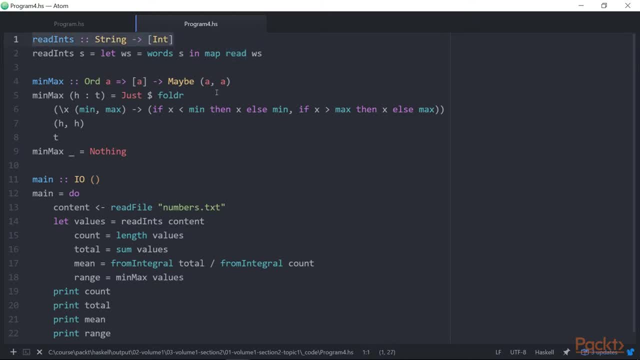 signature up here. This is read as read: ints has type string mapping to a list of int. In min max we use fold R, which we've seen before. We also see just and nothing. Since these are capitalized, we can tell immediately that they are most likely. 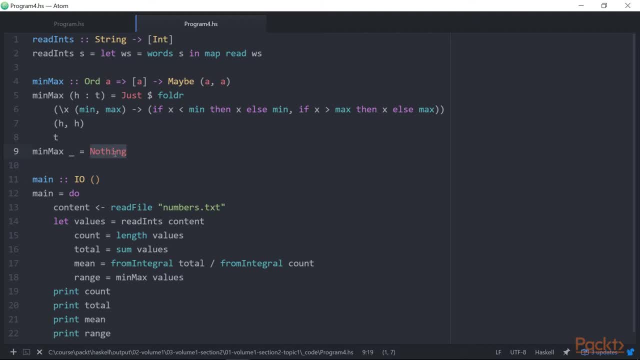 types, type constructors or data constructors, and indeed, in the context of these expressions, they must in fact be data constructors and in fact they belong to the maybe type shown in the type signature. They're used to construct data instances of this type. We can also see that min. 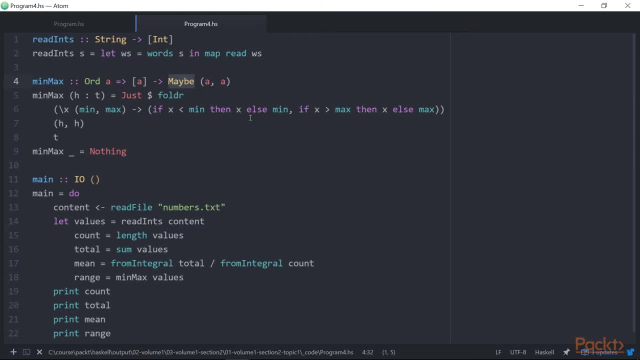 max defines two different bodies or cases which are associated with different patterns of the first argument, which is a list of A. The first body deals with the case that the list has a head H and a tail T. This is the case when the list is not empty. Meanwhile, the second body handles the case of an empty. 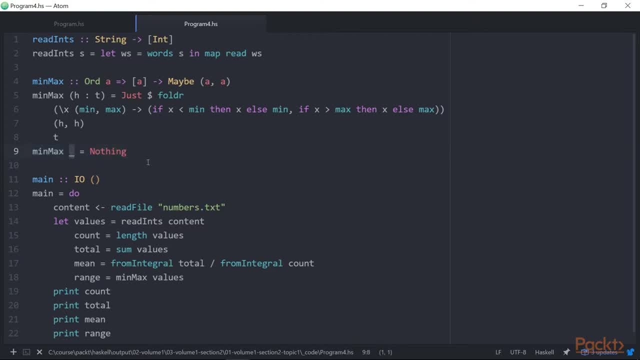 list and we use an empty list. This is the case when the list is not empty. Meanwhile, the second body handles the case of an empty list and we use an empty list underscore to mean otherwise or anything. This matches anything that isn't matched by any other patterns previously given for a function's body. 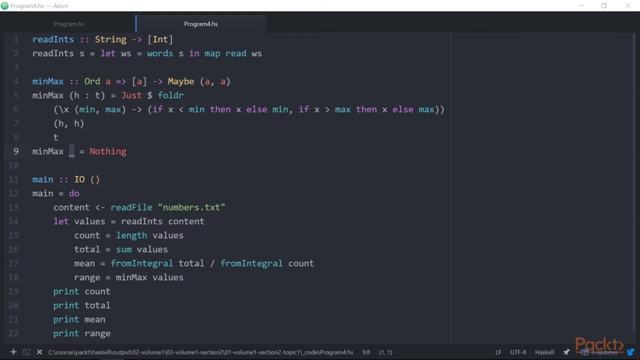 We will go into pattern matching as well as the maybe type in much more detail later. So this function applies fold R to an anonymous function. This is indicated by the backslash, which is supposed to be a rude approximation of a lambda character, and it makes use of parentheses both to construct pairs and 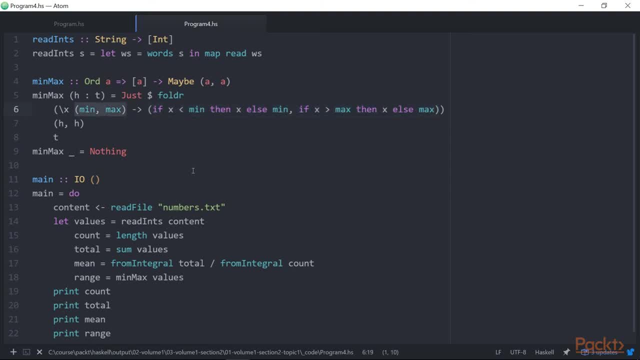 as in this case, and to pattern, match or deconstruct pairs. We also see if, then and else for conditional expressions, We also pass another pair as the initial value to the fold R. This is the pair of two head elements, and then this is also: 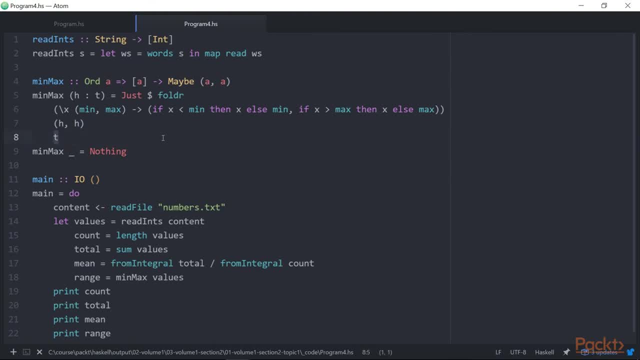 applied to T, the tail, ie the remaining elements of the list. So, overall, this function yields the minimum and maximum values from a list of some ordered type, as long as the list is not empty. otherwise it will return nothing. This is a polymorphic function that can operate on lists of any type: A, for which 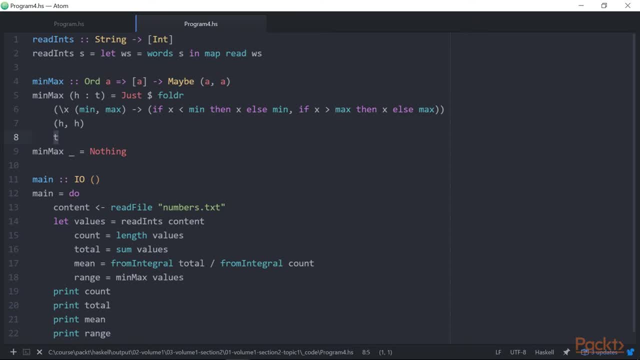 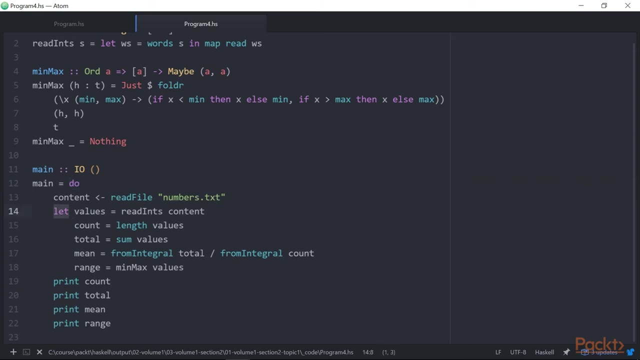 the odd A constraint holds. Odd is a type class that is implemented for types for which a meaningful ordering exists. We also introduce many of our own names in different lexical scopes. so let's look at main. Main also uses do notation and it has another let binding. This let binding, however, is in the context of a do. 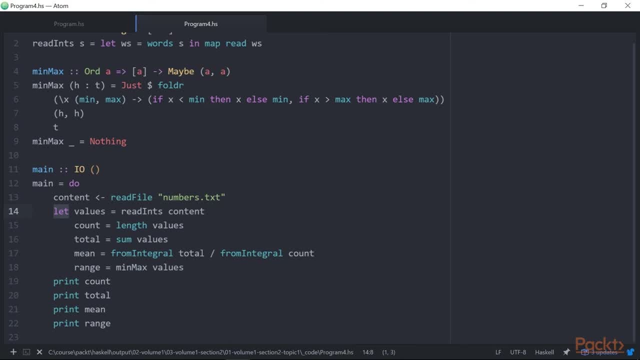 block. In most situations let bindings do not have an in clause. This is because names introduced by let are available from that point onwards to the end of the do block. so there's already an implied scope. Main computes various values from this list of numbers. We read the integers, we get the count of the numbers. 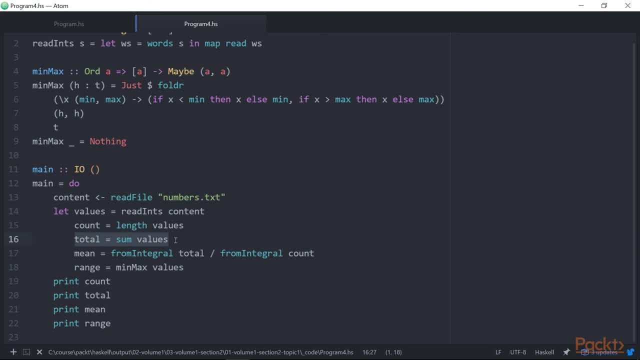 we get the sum of the numbers, which we call total, and we compute the arithmetic mean by dividing the total by the count. It's interesting to note how Haskell handles numeric types: Total and count. both have integral types and integral values and must therefore be explicitly converted from integral before the slash. 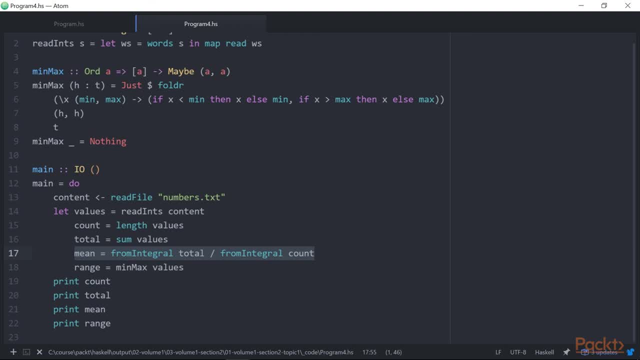 divide operator can be applied to them. This is a good example of how Haskell is always explicit about numeric conversions, and while the absence of the kinds of implicit conversions that the C family of languages and dynamic languages perform is sometimes a little jarring because you have to add these.